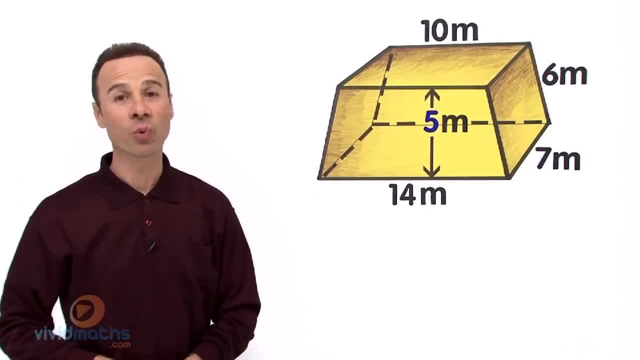 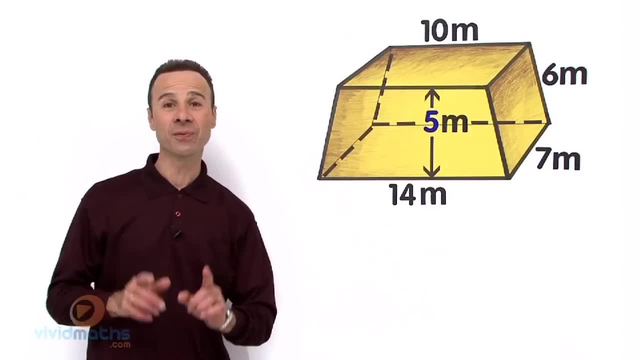 is a trapezium prism and it has six faces, and we are going to do it in five simple and straightforward steps Now, in order to work this out. first of all, we are going to need to find the front face first. Why? Because that is the trapezium part here. See that. 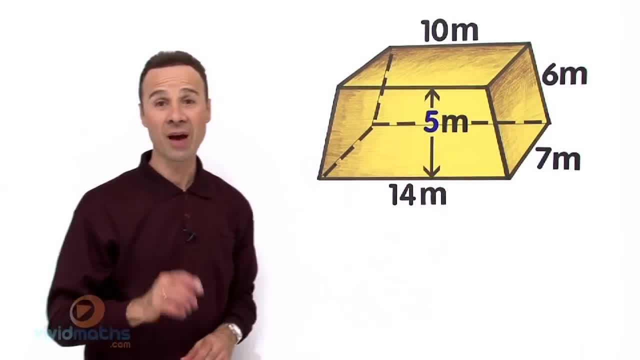 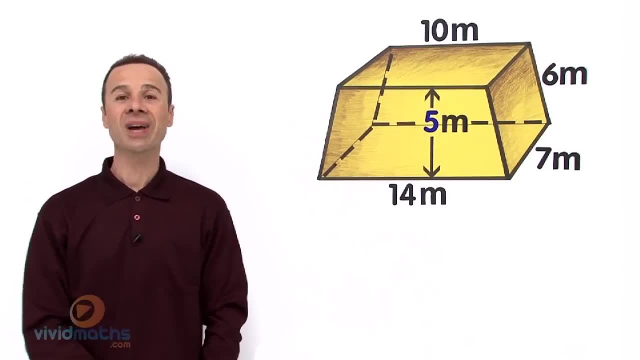 trapezium, two parallel lines and two lines coming out there. We do have a vertical height perpendicular right there, So let us go to step number one Now. before we do that, all units are in meters, so the answer is going to be in meters square. 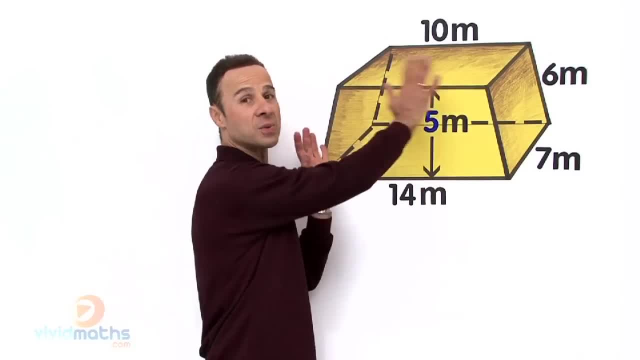 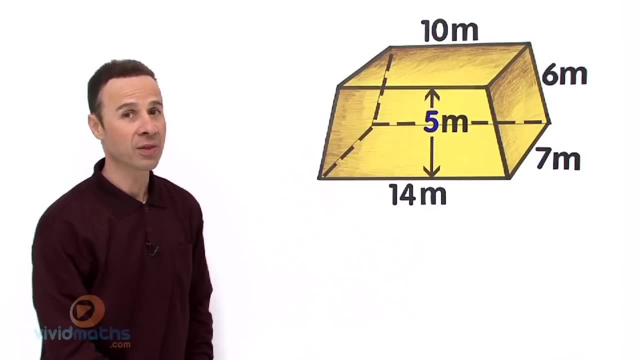 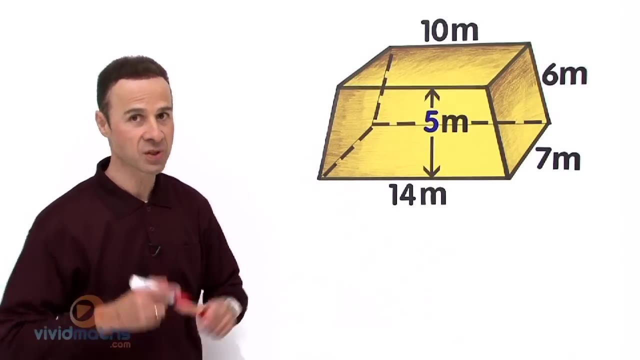 So let us find out the full scope of the entire space all over the skin of this trapezium prism. Step number one, as I said earlier, is to work out the face, this front one here, which is a trapezium. Let us work that out. So the formula for the area of a trapezium: 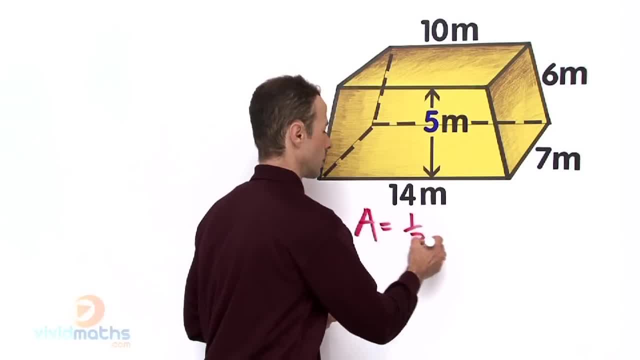 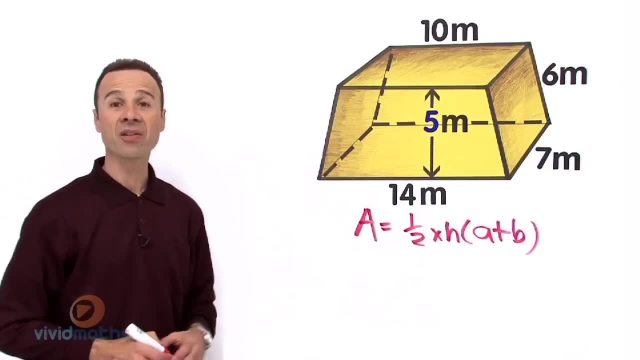 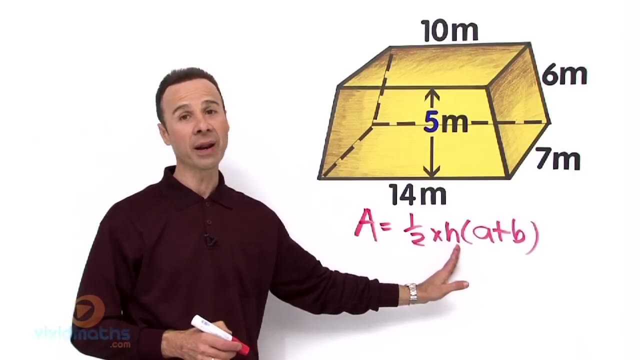 is – if you don't recall it, you may want to revise it from the other chapters, but feel free to watch this now as I go through it in a lot of detail for you. So we got a half times the height. now that height has to be perpendicular height. there is that perpendicular. 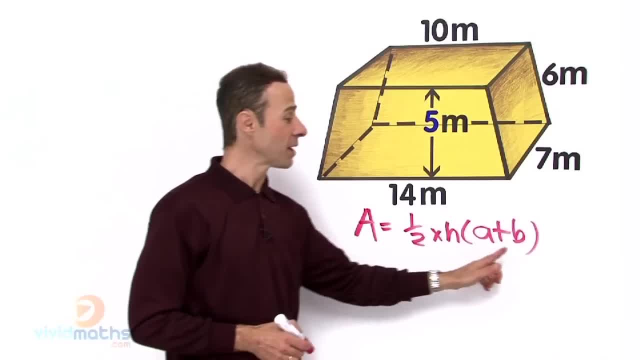 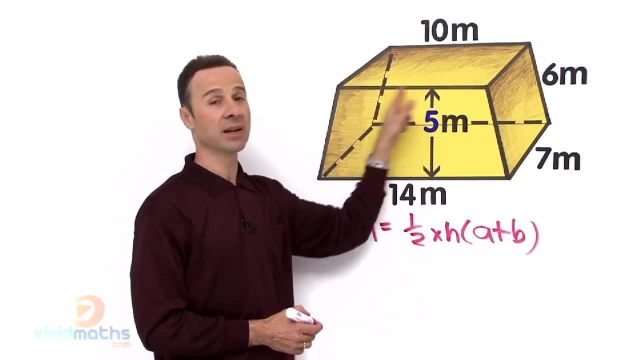 height there it happens to be 5 meters and the A plus B are the two parallel lines top and bottom. We got here 10 meters across here, so if that is 10, that is also 10. here Can you see that That is 10, because that is 10. and down the bottom, here at the base, we have 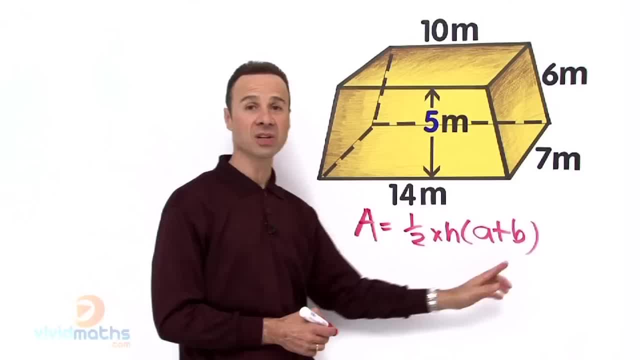 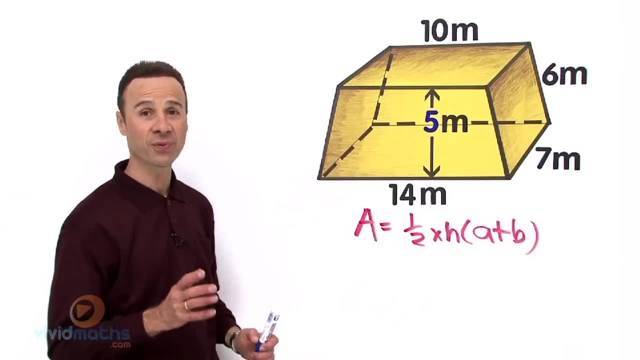 14 meters. So that is going to be A and B respectively. So let us plug in, drag and drop those numbers into the formula so we can work out the trapezium area of the front face. Now, by the way, if the front face comes up to a certain amount, 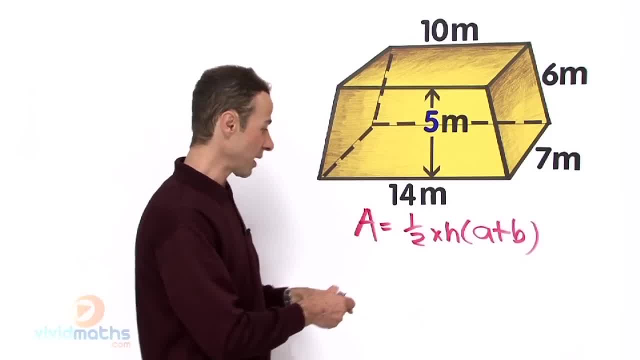 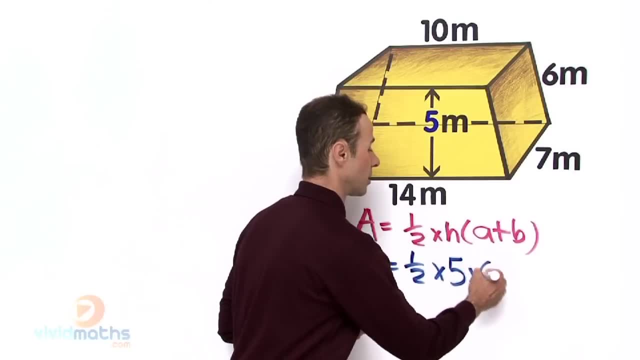 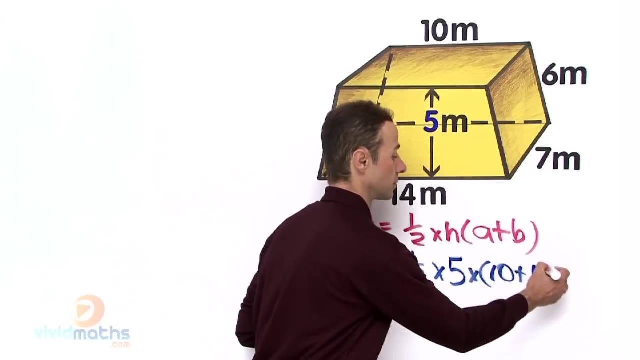 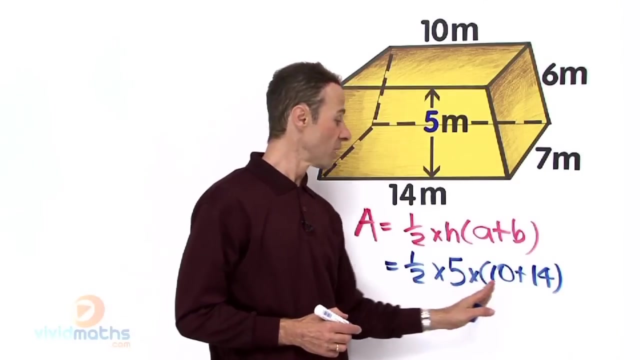 the back face will be exactly the same. So let us work that out. Vertical height 5, A across here is 10 and B the base is 14.. Ok, let us plug that in now in the calculator. so it is going to be a half times 5, which is 2.5 times 10 plus 14,. 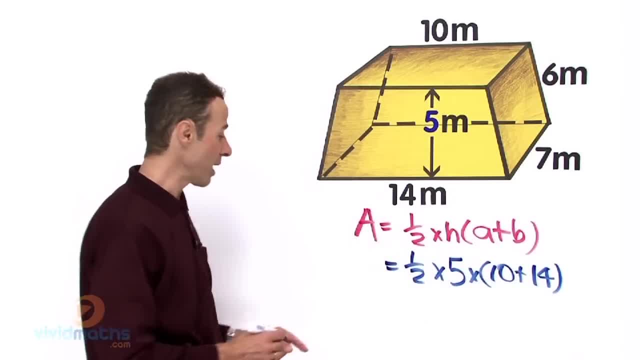 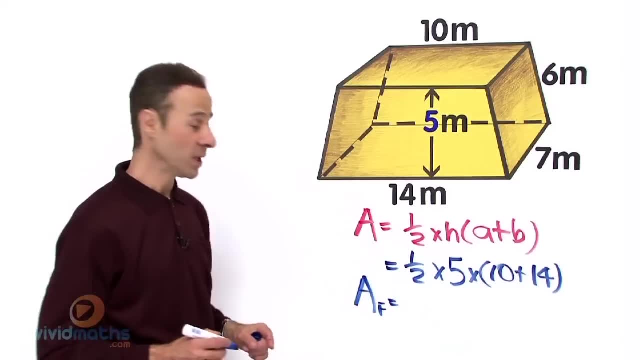 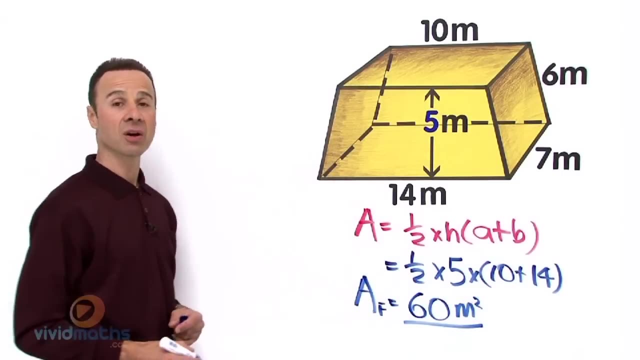 10 plus 14 is 24.. So multiplying all that throughout the area of the front face all together on your calculator is going to yield 60 meters squared. Ok, that is the front face, which means the back face is going to also be 60 meters. so let us put area of back. 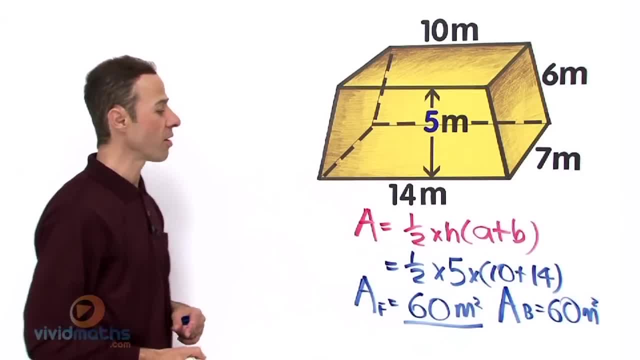 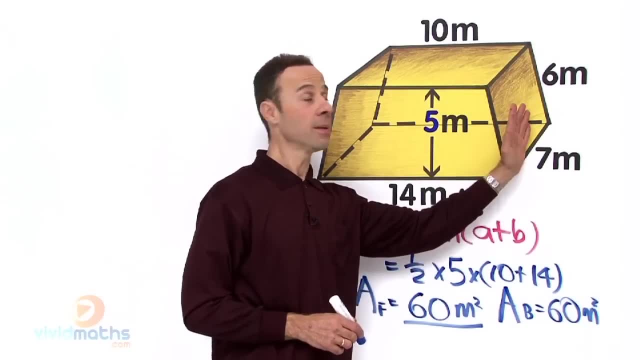 Ok, there is the area of the back. we got the front and the back. Now where we go is to the right side face, and the right side of the face is right over there. We can see the slant length. there is 6 meters and the depth is 7.. All we need to do now is length times. 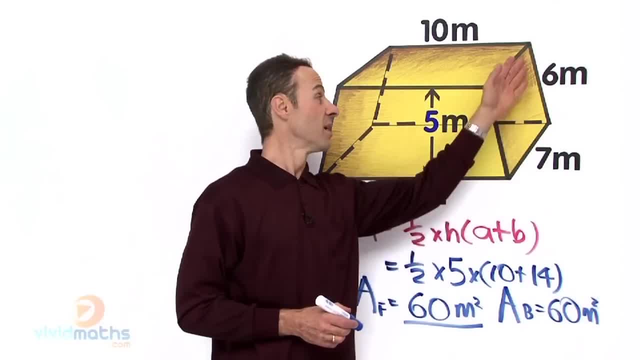 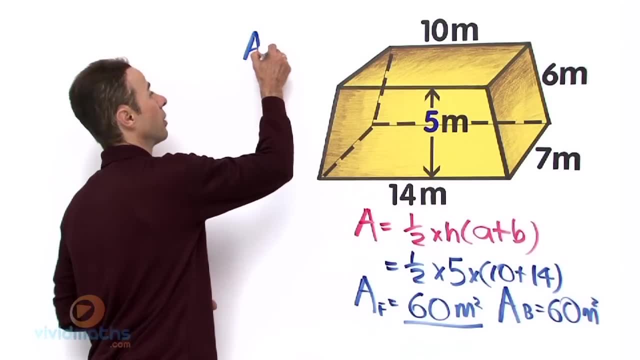 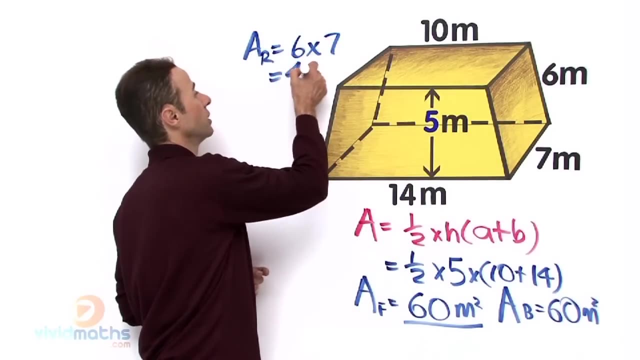 breadth and work out that simple area of that rectangle right there 6 times 7 is 42.. So right side of the face, area of the right equals 16.5 meters 6 times 7, which equals 42 meters squared. so there is the right side. Now, if the right 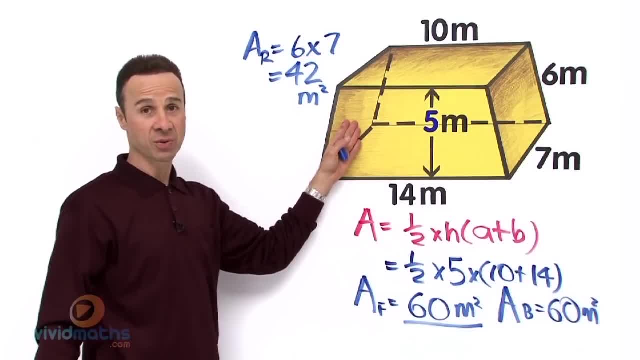 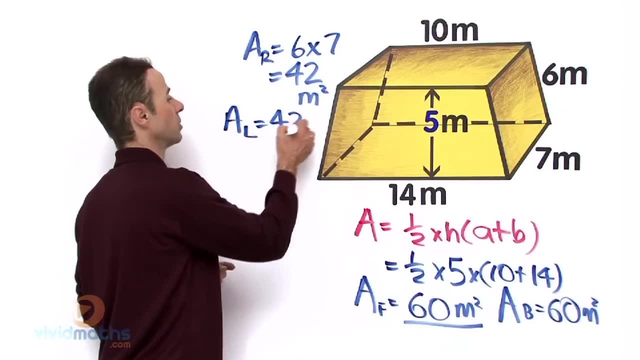 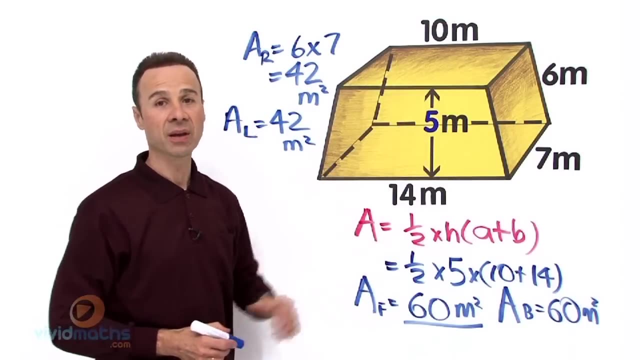 side is 42. guess what? The left side, because it is symmetrical, is exactly the same, so that is also going to be 42.. So area left equals 42 meters squared. So we got the front, we got the back, we got the right, we got the left. Now let us work out the area of the. 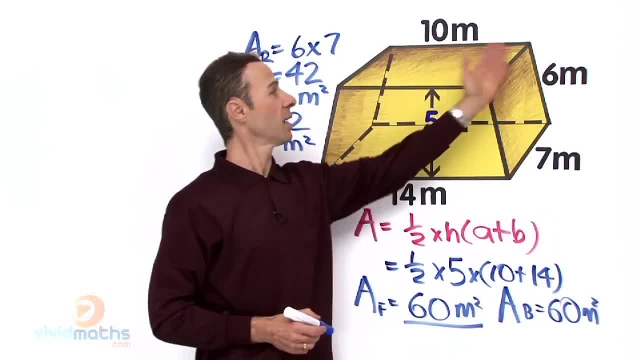 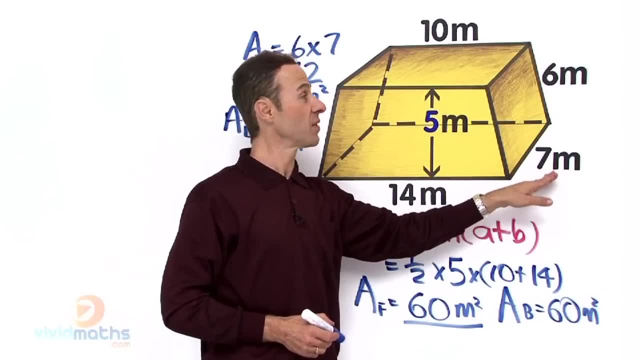 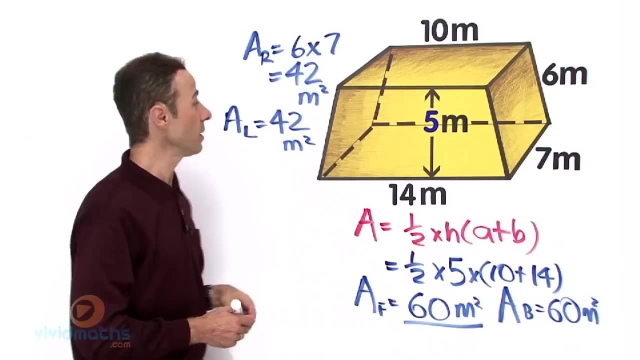 top right up there. So what is that area? Well, that is going to be 10 across there times the depth. there It is going to be 10 times and the depth is written right there. so that is 7 there, that is also 7 there. So 10 times 7 that is going to give us 70.. So that is the top face there. 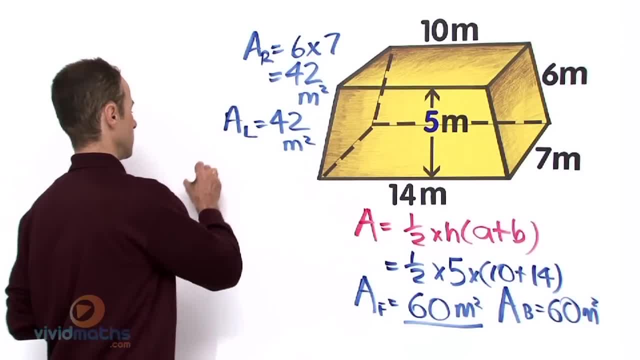 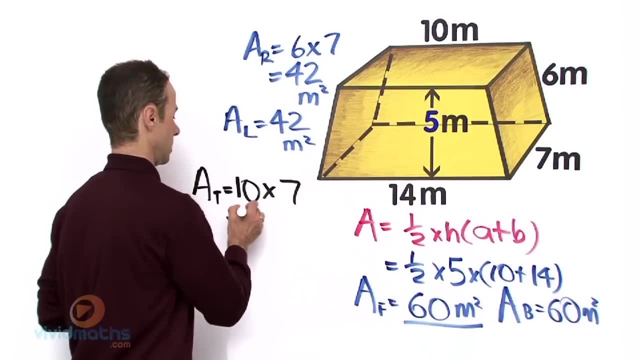 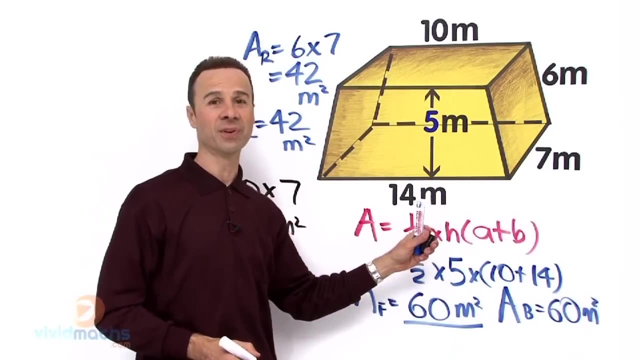 So area of top? Ok, Now, if the area of top is 70 meters squared, is there at the bottom? No, it is different, is it not? Let us have a look here. The area of the bottom is 14 across there, and the depth 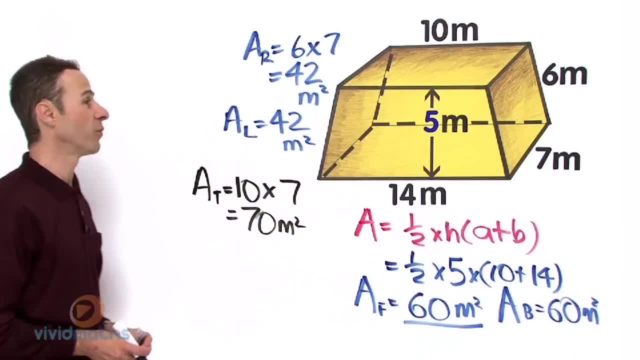 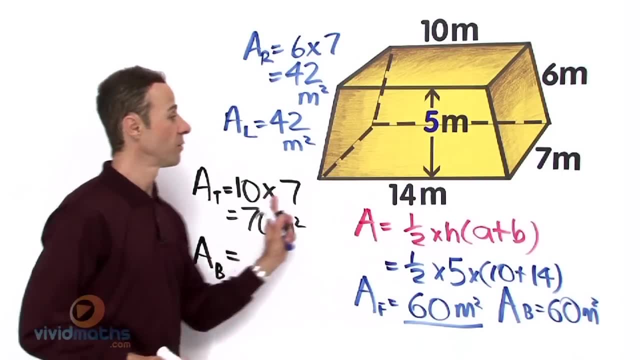 is 7 across there, so that is going to be 14 times 7. so area of B- B for base or bottom equals 14 times 7. And that yields a total of 14 times 7. is that amount? Congratulations to you. 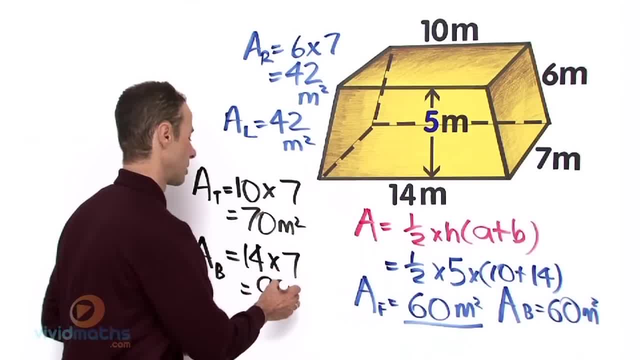 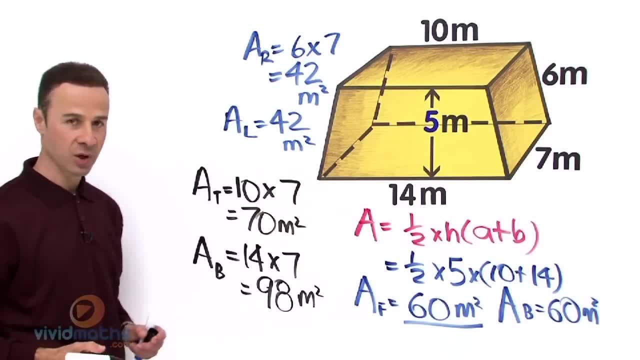 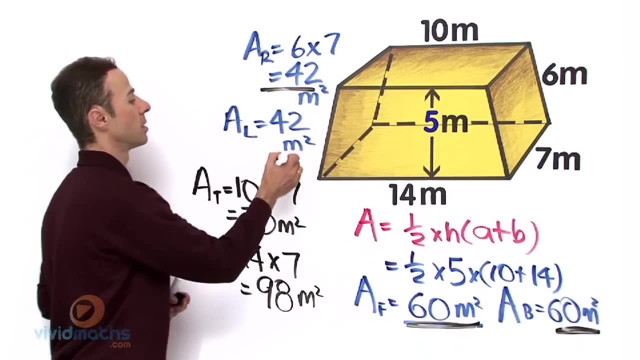 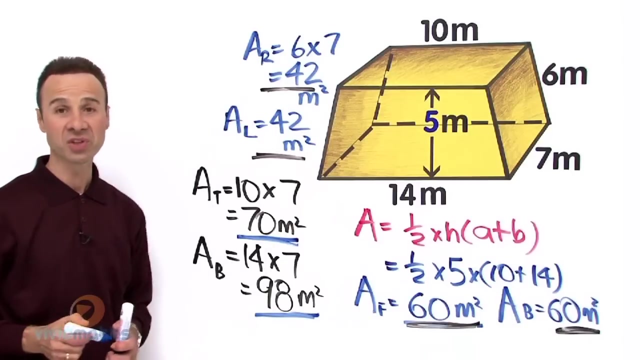 Thank you, Thank you. seven is ninety eight meters squared. Now we have worked out six faces. let us check that. we got six. we got one, two, three, four, five and six. therefore, we have all six faces. all we have to do now is add them all together to get the complete space surface space of 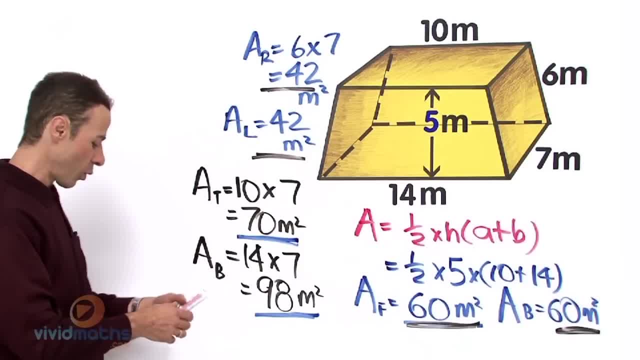 this and surface area of this trapezium prism. so let us add them all together. So we have the two sixties, which are the areas of the front face and the back face. so let us write that up. and then we have the two forty twos, which is the right face and the 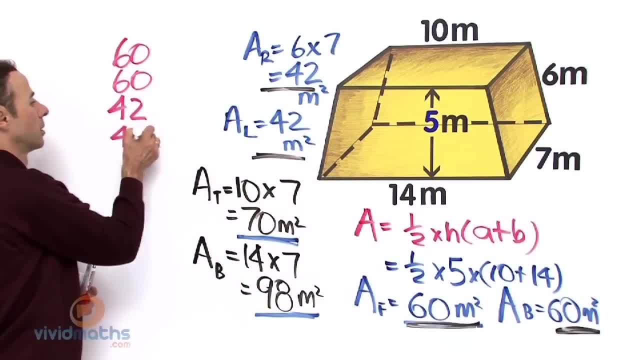 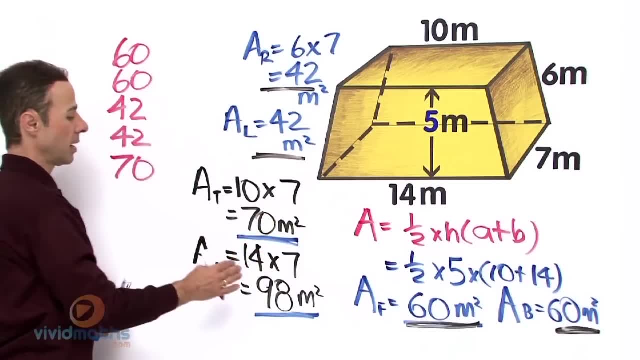 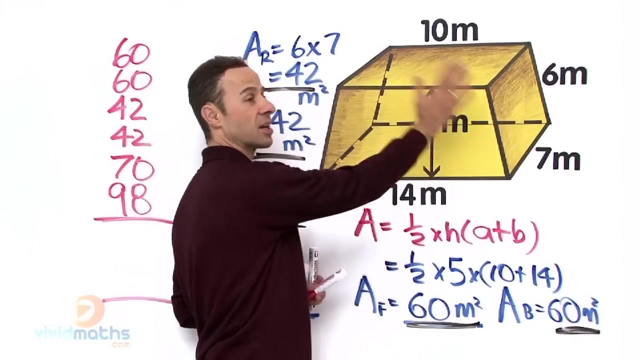 left face, And then we have finally the top, which is up there, which is seventy, and the bottom, under there, fourteen times seven, which is ninety eight. Ok, let us get our calculators out so we can work out the total complete and scope and size of the skin and the exterior outside surface of this trapezium prism. 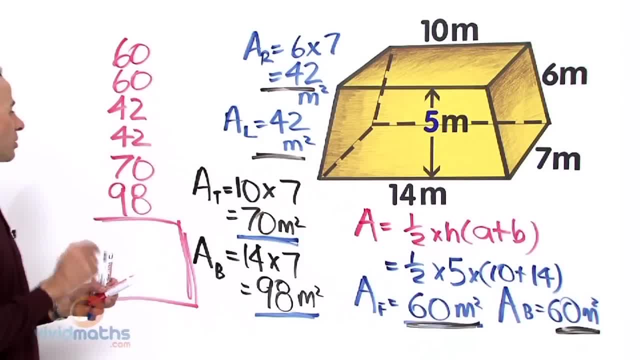 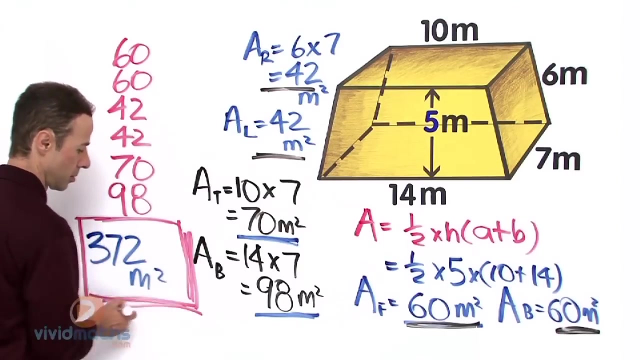 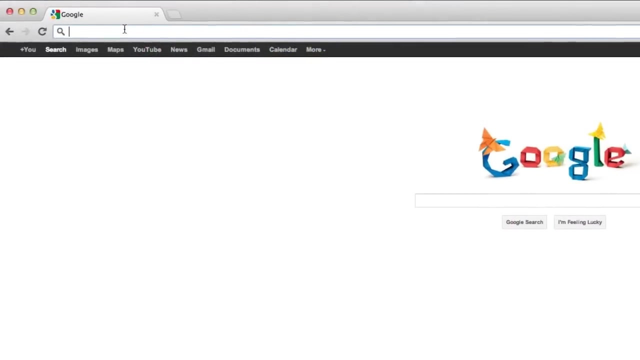 So in our calculators, sixty plus sixty plus forty, two plus forty, three plus forty, three plus forty two plus seventy plus ninety, eight, altogether grand total, the entire total, complete surface area is: Take a minute to check out our website at http//wwwyoutubecomau and go to our website. 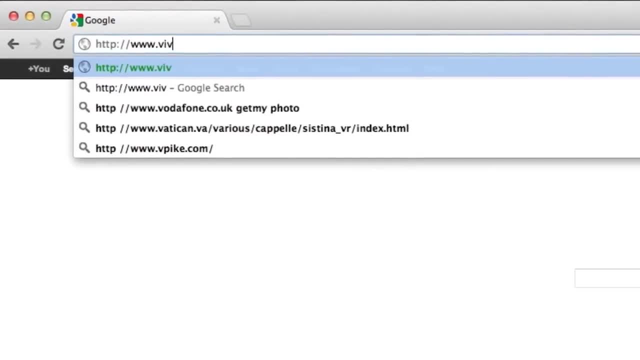 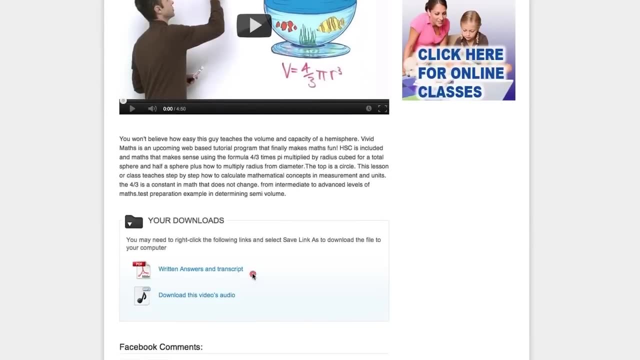 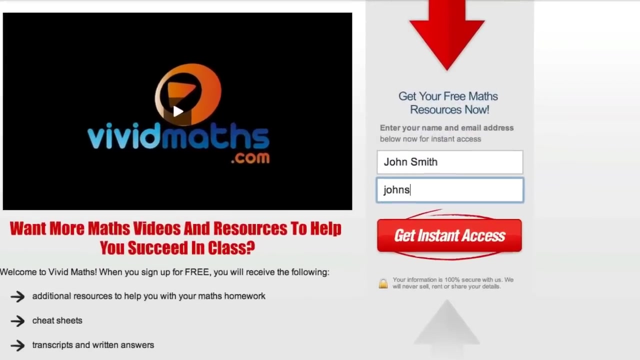 at http//wwwvividmathscom, You will find additional resources, cheat sheets, transcripts and other math videos that are not available on Youtube. Lastly, don't forget to subscribe to get access to all the written answers for your math questions, plus other special offers.